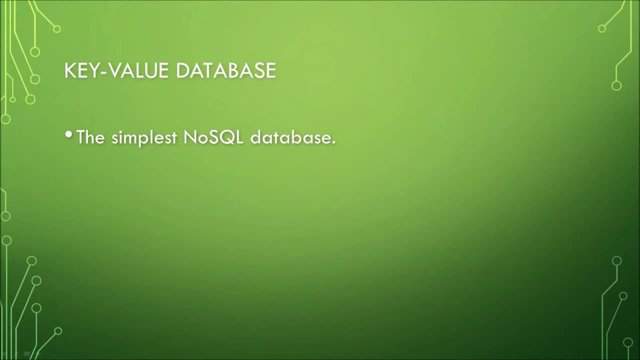 Now the key value database is the simplest NoSQL database wherein every single item in this database is stored as an attribute, name or key together with its value. So there's a key and you will get a matching value. You can have another key and you will get another. 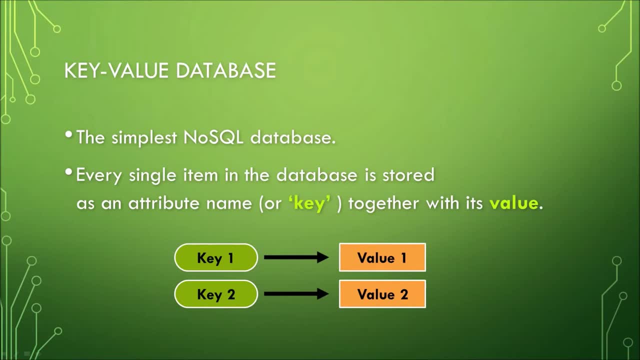 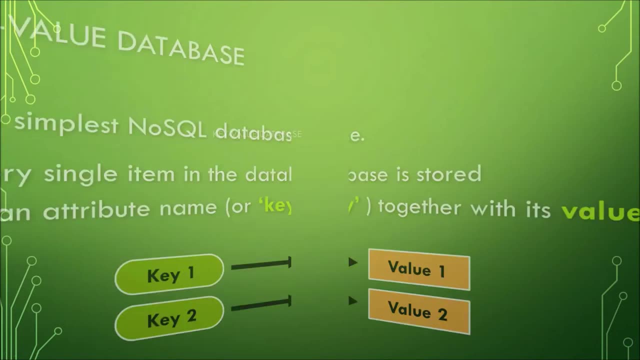 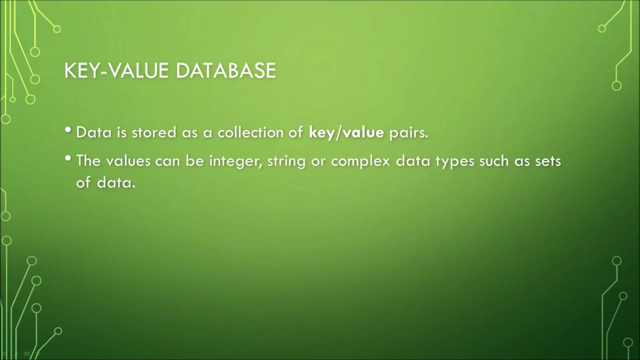 associated value. Again, there is a key and a value. If you have a key, you will then get its associated value In a key value database. data is stored as a collection of key value pairs. as what was emphasized earlier, The values can be integer, numbers, a string. 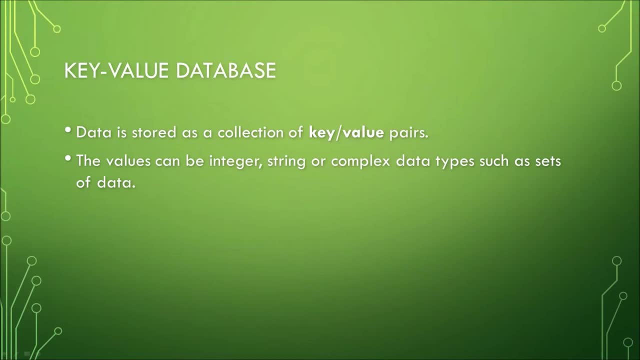 names, address or complex data types such as sets of data, and it can be files or videos, The exact match, if there will be duplicate keys, right. So in key value databases, keys must be unique. Now, to retrieve data, you must have the exact key, So data is retrieved. 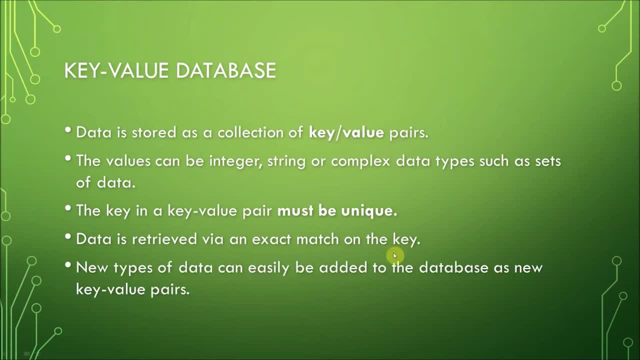 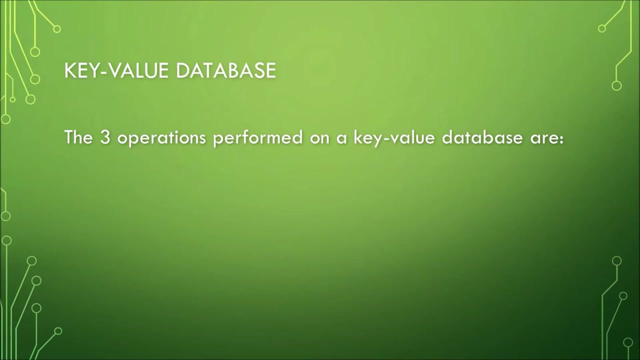 via an exact match on the key. Now, one advantage of key value database is that new types of data are added to the database as new key value pairs. And with this, here are the three operations performed on a key value database. The first operation is PUT. PUT adds a new. 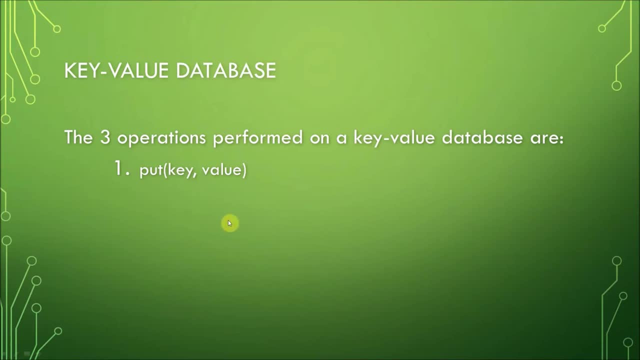 key value pair. As you can see in here, PUT adds a new key value pair. You pass a key and a value to the table, Or PUT can also update a value if this key is already present. The next operation is GET. Now GET returns the value for a given key, if it exists. So 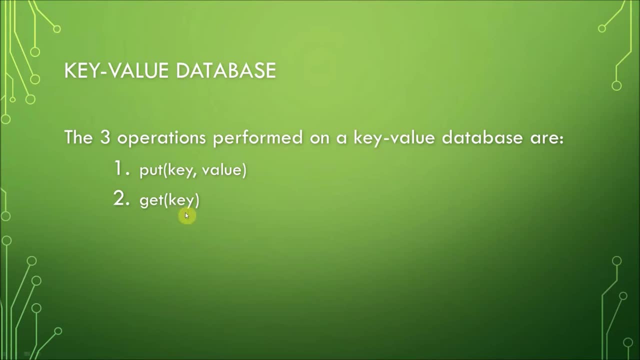 we pass a key and then we will then get a value with that associated key. The next operation is the DeLTE operation. So DELTE here removes an associated key. So DELETE here removes a key and its value from the table if that key exists. so we pass a key and once it is, 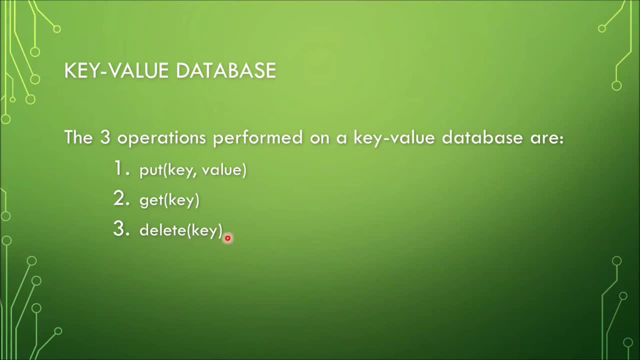 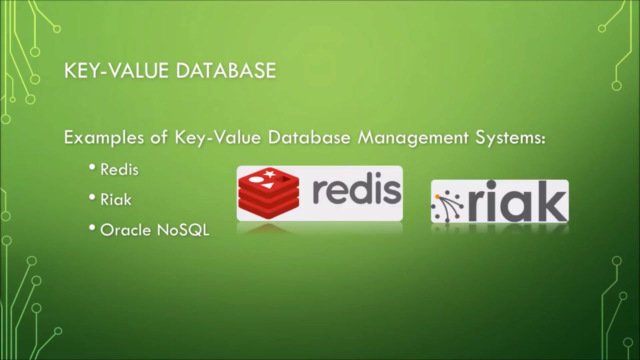 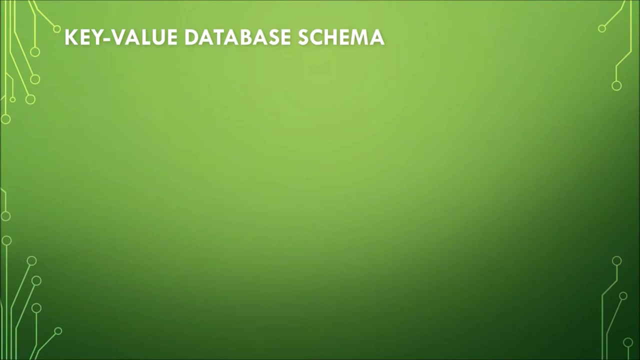 found in the table in this key value database. it then removes the key and its value. now now here are some examples of key value database management systems. we have Redis, react and Oracle, no SQL, and there are also other database management systems for key value databases. so how do we make a schema for a key value database? here is how consider the student relation given. 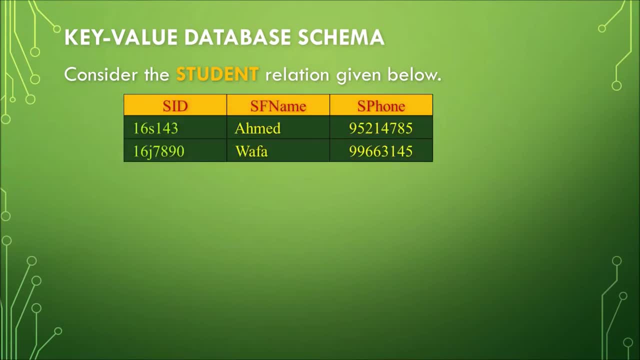 below. so this is a student table and it has three columns or three fields or three attributes, and this table are related to the table and this table are related to the table. and this table also has two rows or two records: one record for the student named Ahmed and one record for a. 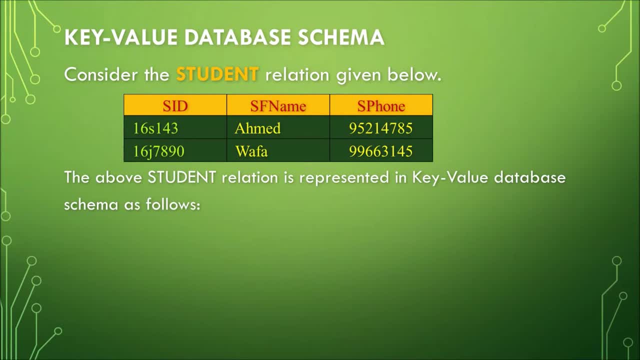 student named wapa. now the above student relation is represented in key value database schema as follows. so here is how it is being done in a key in a key value database schema. this is: this would be the new structure in a key value database schema. these two entries here are common. 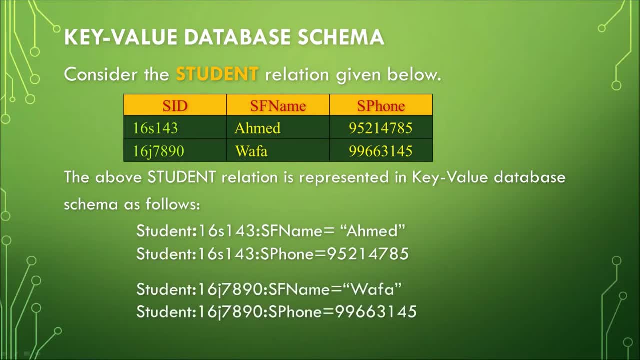 from this first record. the next two is based on this record here. the first record about waffle. now let's get into the parts of this schema. the first part in this schema is the key and obviously the next part would be the value. thus, key, value, database. right, the key is kind of a. 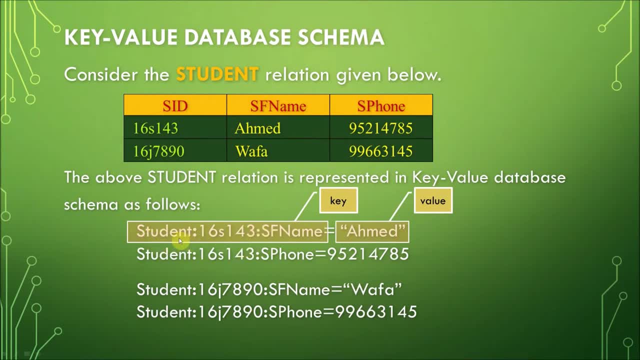 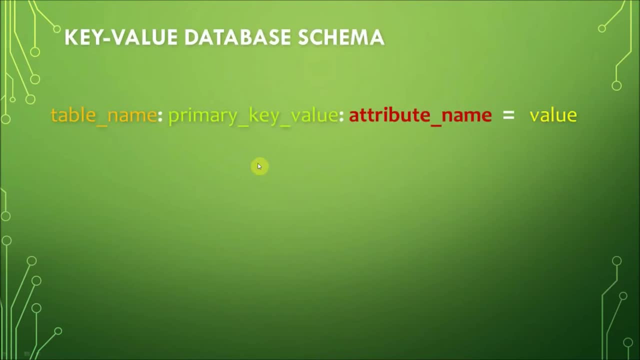 complex. it's not an ordinary key. as you can see, there are parts right this. you might have an idea already as to what this one is right. so let's get into the parts of the keys and then also the values. so the first part of the key is the table name and then you have the colon symbol, Colin dot dot. 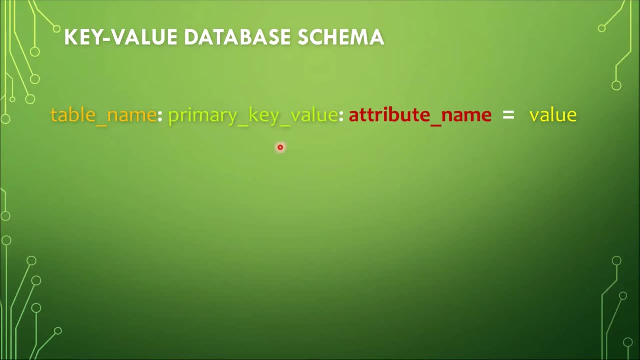 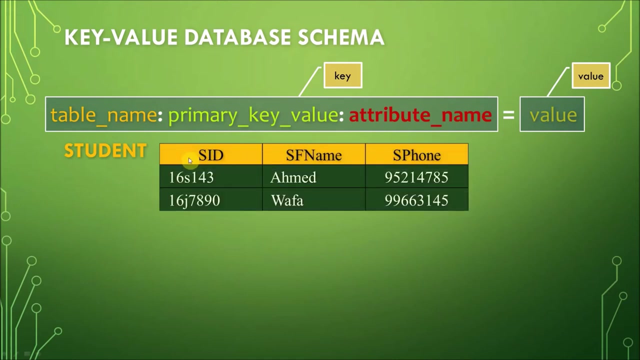 and then the primary key value form for a record, for one record and then a column and then the attribute name. so this will form part of the key. the next part here is the value. you have here an equal symbol and then the value, so key value. now let's consider again. 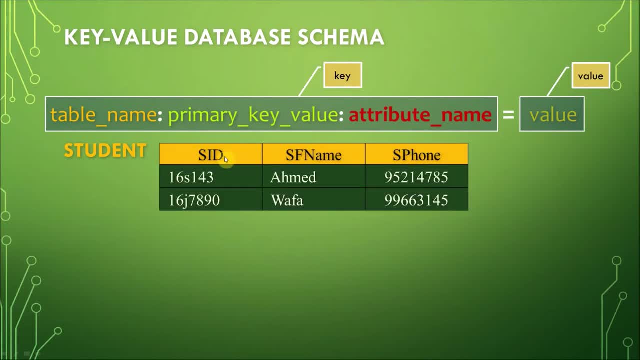 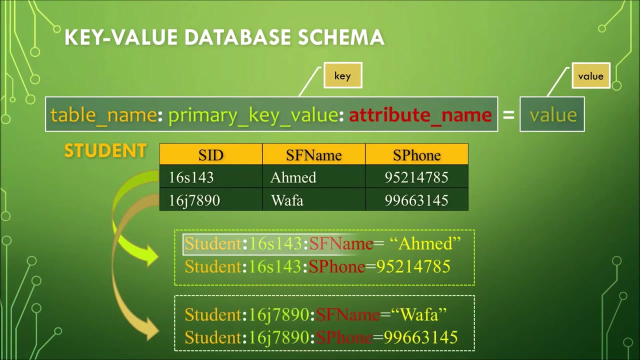 the student table, the one that we have in the previous slide. so here is how we convert to the first record. we will have two entries for this, one, okay, and the next record, another two. this part here is a key and the next part is the value. okay, so in this key value pairing, in this key to 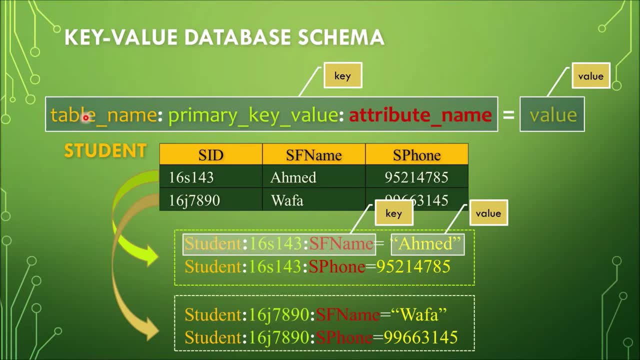 be specific in this key: student refers to the table name. so here we know that this is a student table. so this is the name, table, student column and then primary key value of the first record. so the first record is one, six s, one, four, three. so we follow it and put it here: colon, and then the first attribute or column or field. so 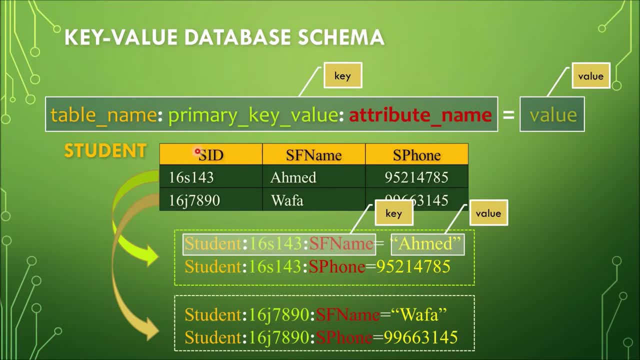 the first column or field here is SF name. we no longer include s ID because it's already here. okay, we just put the non key attribute, so we start off with SF name here. so this will form part of the key table name: primary key value and then the attribute name. 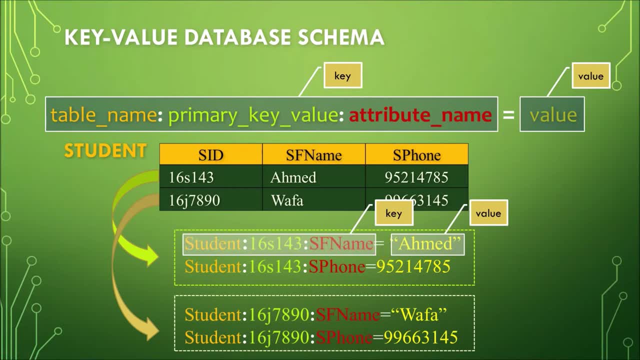 again. this will form the key and then you have the equal symbol and then the value. so the SF name of student one six s, one four three of the student table is a man. this is the value: a man. notice also that double quotes are placed in here because 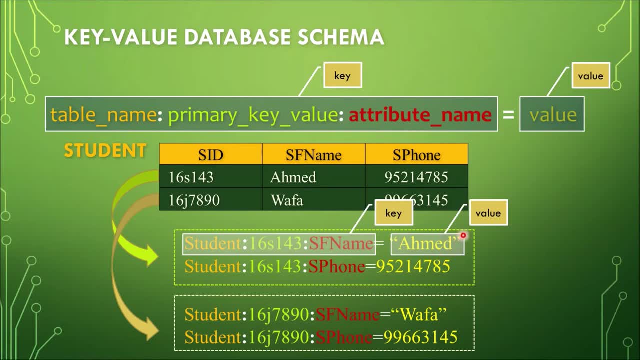 Ahmed is a string, and strings are enclosed inside double quotes, double quotation marks. okay, now this is the next entry. this one is still 4, 1, 6 s, 1, 4, 3, 4, Ahmed, but this time the attribute is phone s, phone for the phone. we're done with the SF name. we're done with the first name. let's go ahead with the. 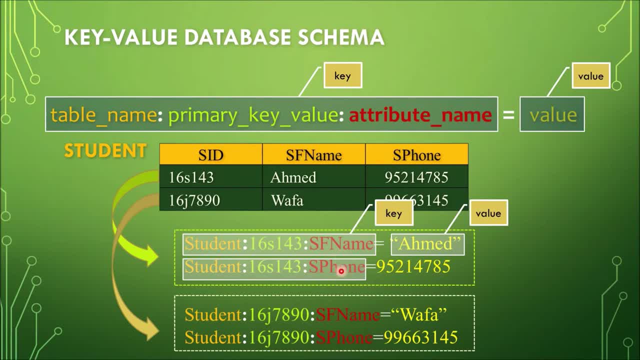 so table name, primary key and the next attribute, which is s phone, and then that forms the key and this would be the value. the value for Ahmed's phone is nine five, two, one, four, seven, eight, five. this is for the phone of one, six s, one four, three. now for the next record here. know this same. 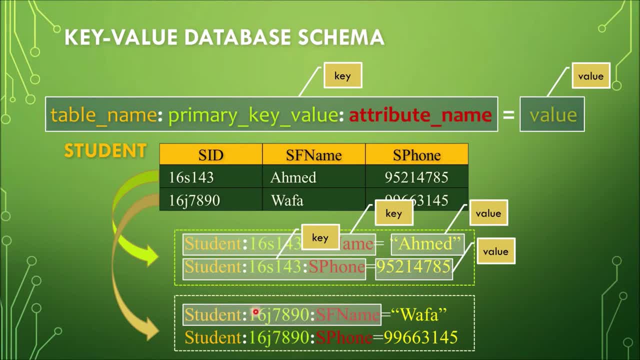 student table, but this time a different primary key, because this next entry here refers to the second record in the original relational schema in here. so we have one, six, J, seven, eight, ninety for the second record, and then we follow again the attribute SF name. again no SID here, because 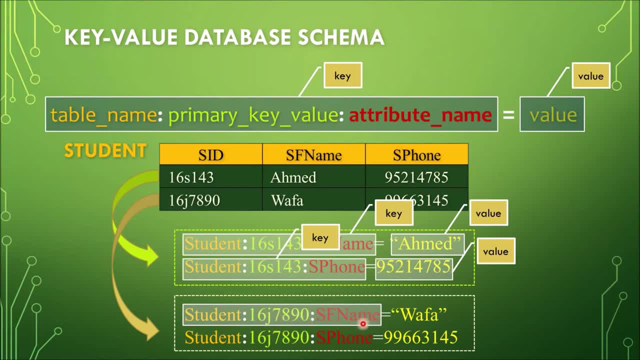 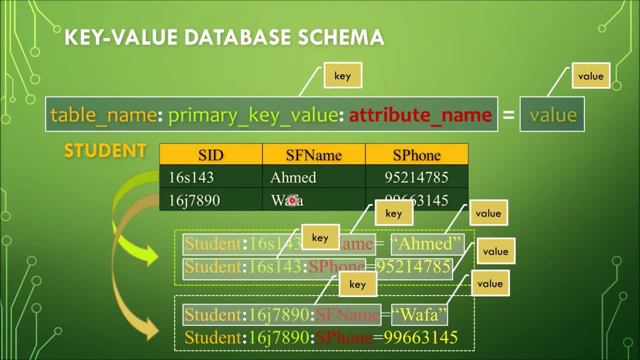 would be WAFA. so we have here WAFA as of name column. the students first name of student 117 j 7 890 in the student table is WAFA. the second entry here is for the student's phone number of 1: 6 students phone number. 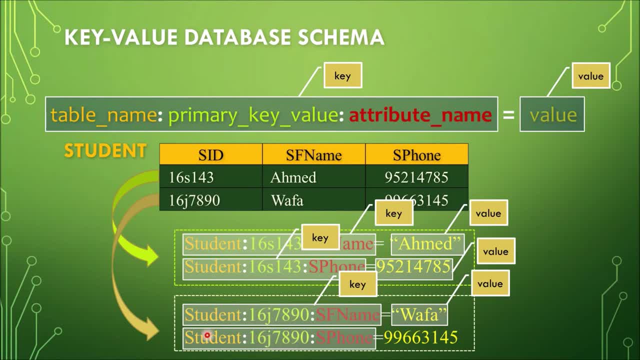 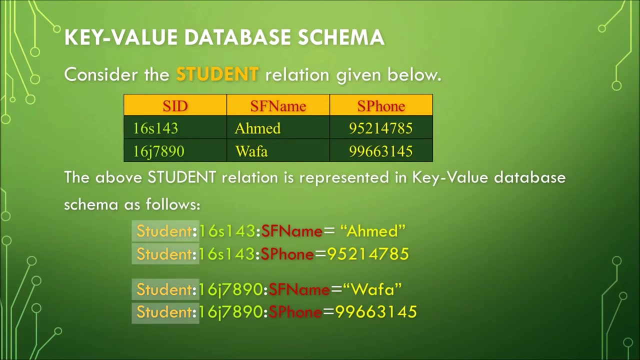 of 1, 6, J, 7, at 90 here and in the student table. so the value for that one is nine six, six, three, one five, nine six, nine, nine, six, six, three, four, five. okay, again, the first part of the key is the table. so you have here the table, student table. the next part of the key is the primary key. so 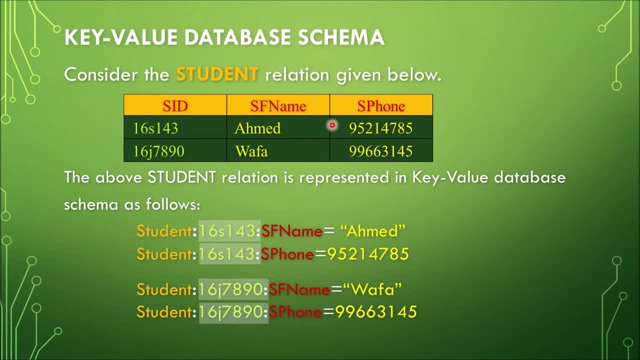 these two here. these two entries refer to the first row and these two entries here refer to the second row, or the second record. as you can see, this is 1 6 s 1 4 3 here and 1 6 s 1 4 3 here. but 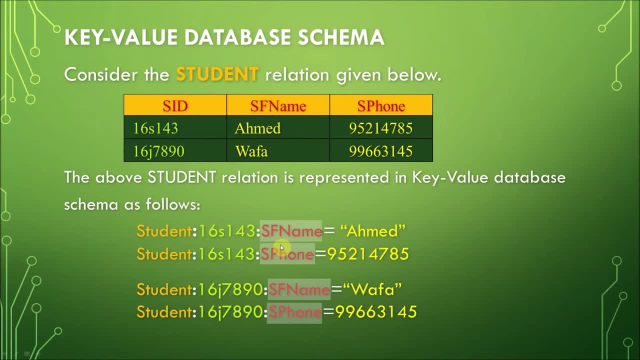 they have different attribute names. so the first entry related to the first record here is attributes name is SF name and the second one is for the for the phone for the students phone. so those are the attributes and this is the value I met is the first name of 1, 6 s, 1, 4, 3. 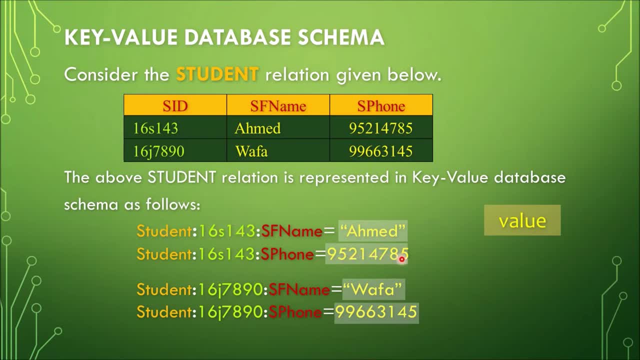 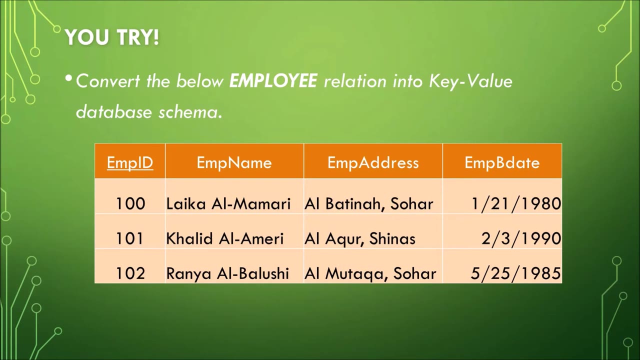 in the student table: 9, 5, 2, 1, 4, 7, 8, 5 is the value of the students phone of 1, 6 s, 1, 4, 3 in the student table. now I want you to try to convert the relation given here. convert the below employee. 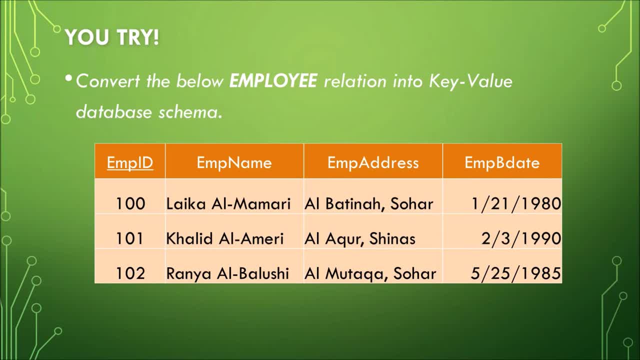 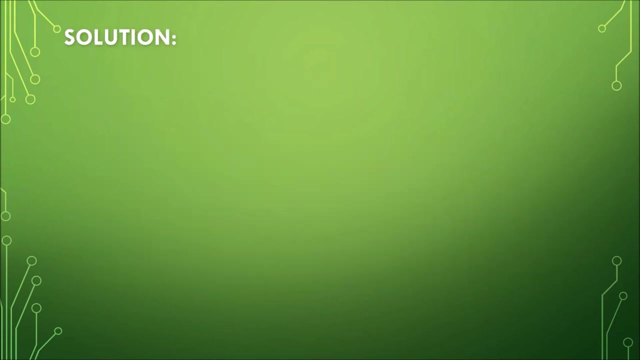 relation into a key value database schema. so this relation here, or table, has one, two, three, four columns and one, two, three records. so I wanted you to try to convert this table with this relation into a key value database schema. so pause this video for a while and try it. so are you done? let's see the solution. did you get this? 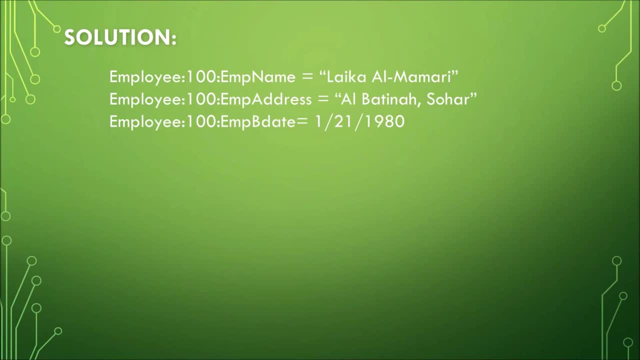 one correctly. this is for the first record. this talks about employee table, employee number 100, column amp name, and then the value is like a alma-mari again. another entry would be for employee 100, but this time for the employee address column and the value is albemarle. 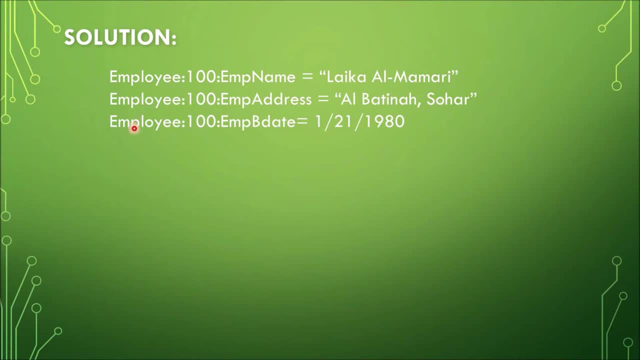 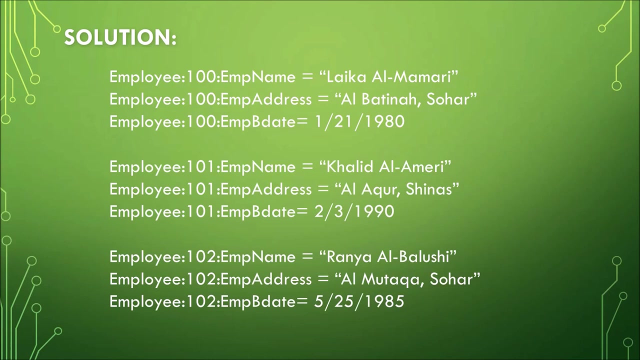 Tina Suhar. then another entry for employee 100, but this time for the employees birth date, which is a value of 121, 1980. and so goes for the next record and for the third one. again, this part is the relation name, Colin, followed by the primary key, Colin, followed by the attribute name, and then